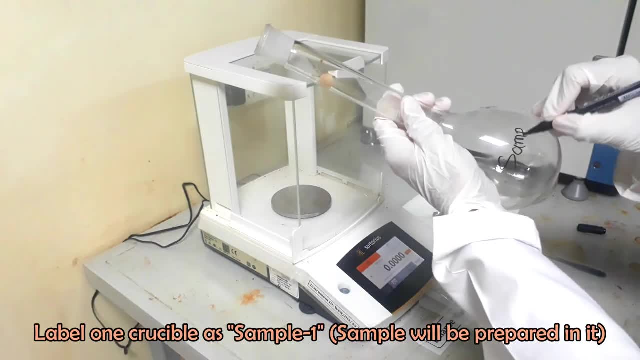 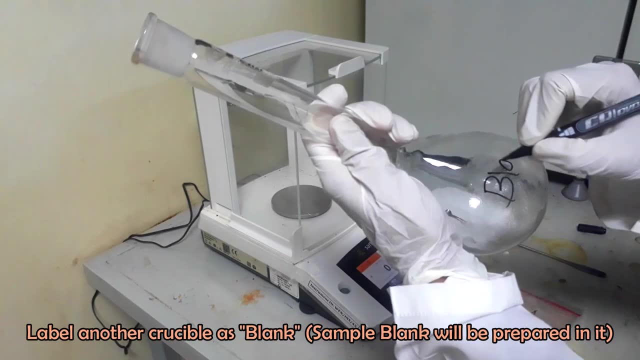 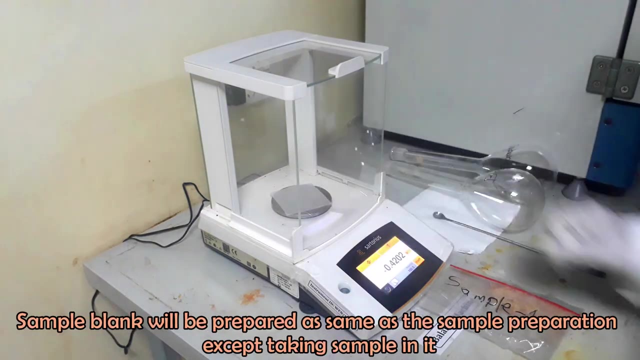 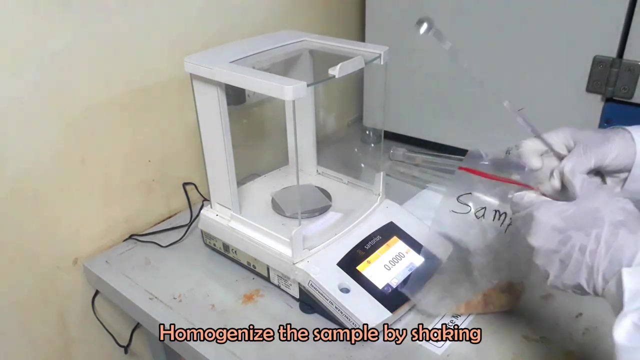 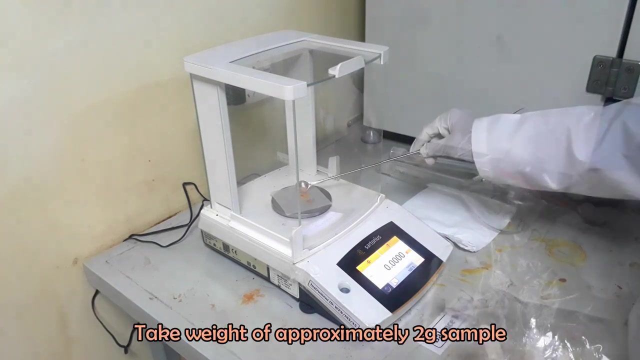 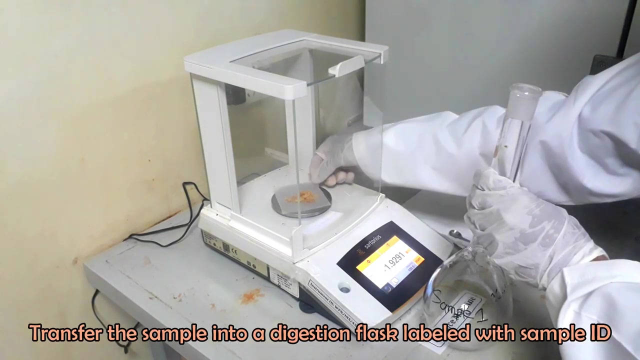 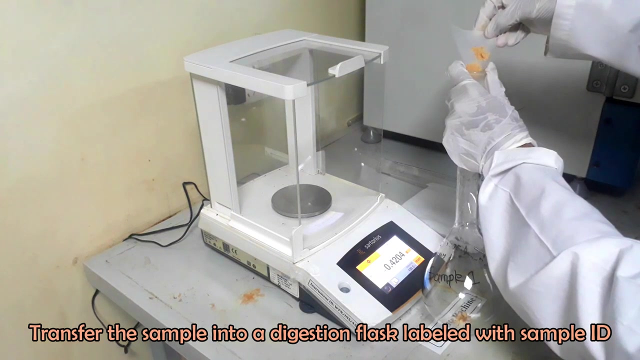 Bring two properly cleaned and dried flasks. Label one flask with sample ID. We will prepare sample in it. Label another flask with blank. Take weight of about 2 grams of sample. Take weight of about 2 grams of sample. Transfer the sample into the flask labeled with sample ID. 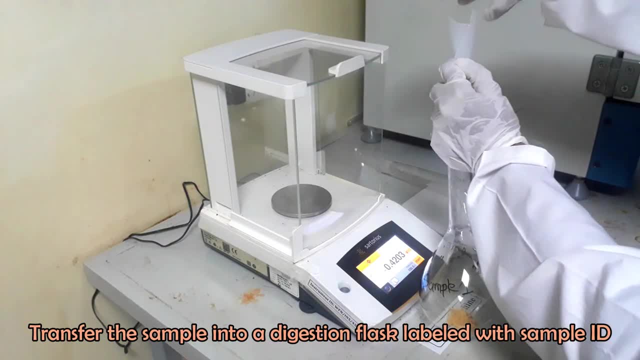 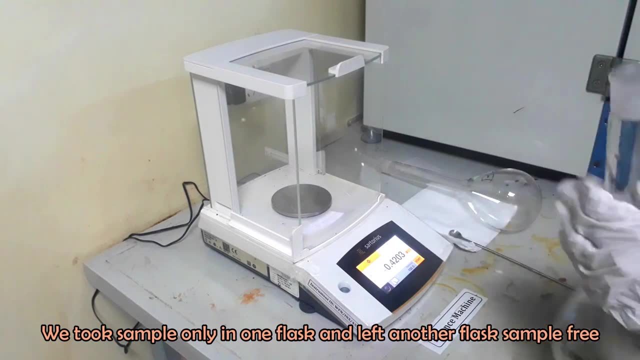 Blob by series of 200 Delta Flask inbank and 25 Delta Flask with a became defective. We took sample in one flask, keeping another flask left blank. We will take sample blank prepared in this blank flask in news page Musik. We took sample in one flask, keeping another flask left blank. 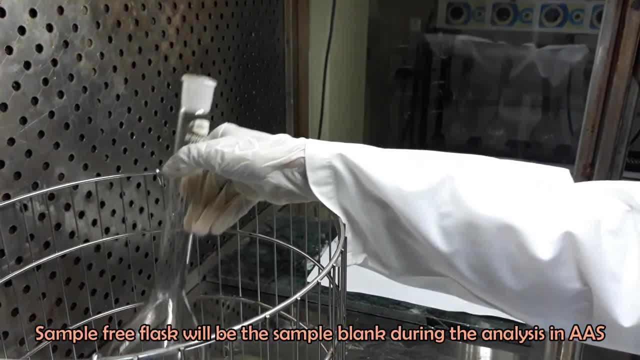 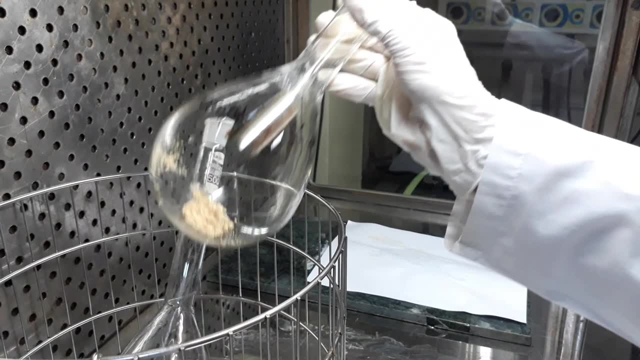 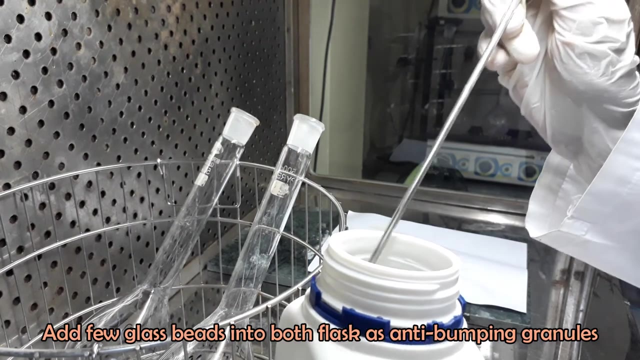 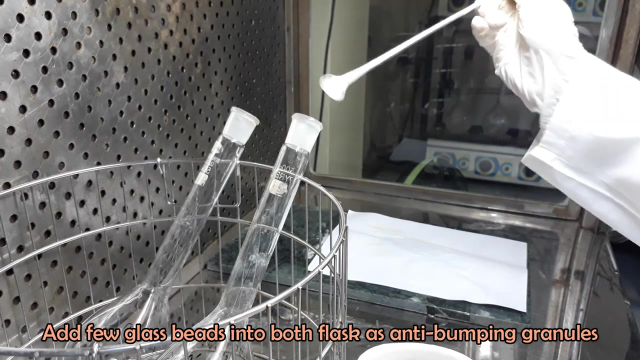 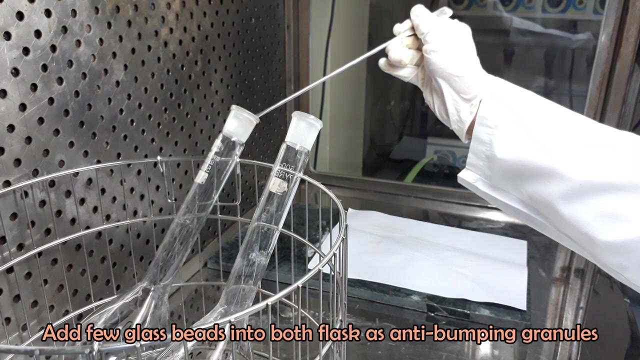 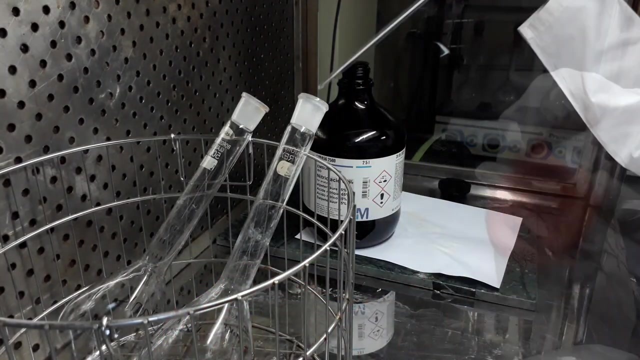 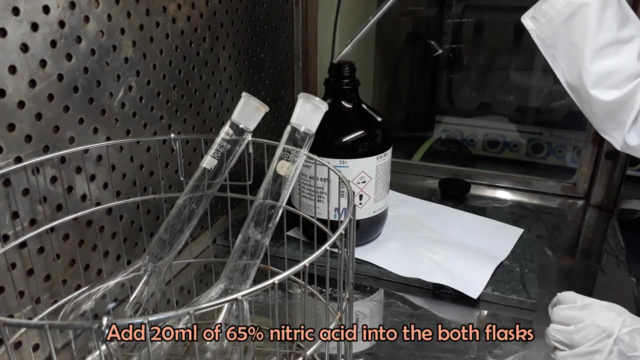 Branding Most Wanna Some비 uds less following every steps for the sample preparation except taking sample in it. Add few number of glass bits Now. add 20 ml of 65% nitric acid into both of the sample flask and blank flask. Now add 20 ml of 65% nitric acid into both of the sample flask and blank flask. 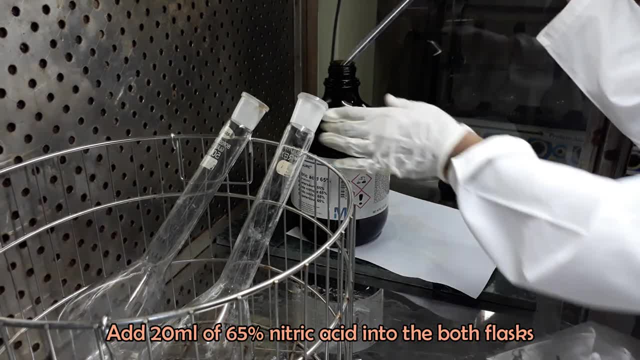 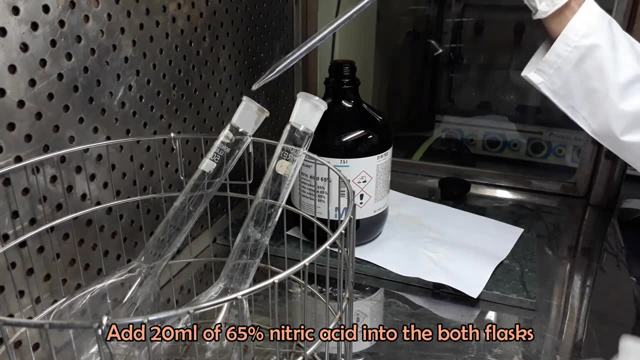 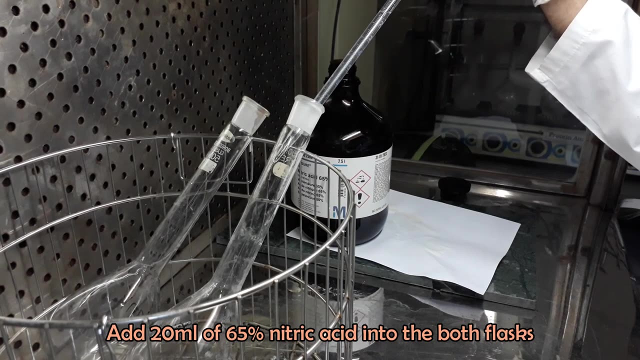 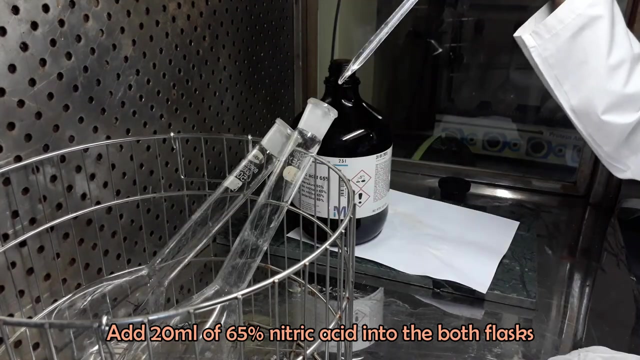 Stir law position has to be safe. Now add 25 ml of씨-isomaldehyde into this small glass flask. Stir. once the mixture being heated, Stir it quickly using down and use a good speed. Repeat on the other side. 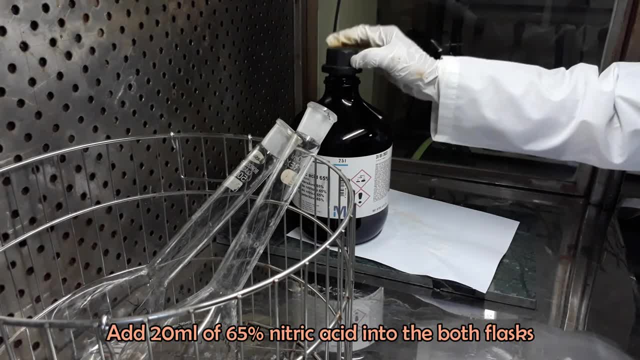 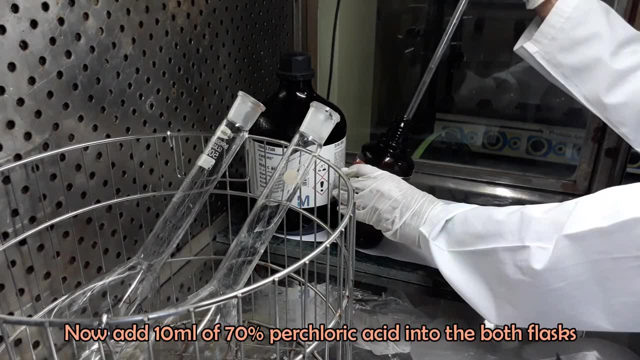 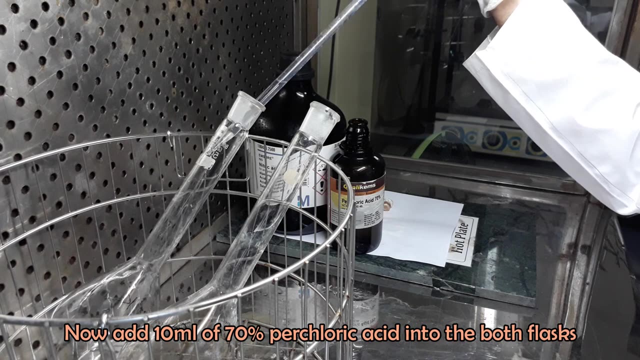 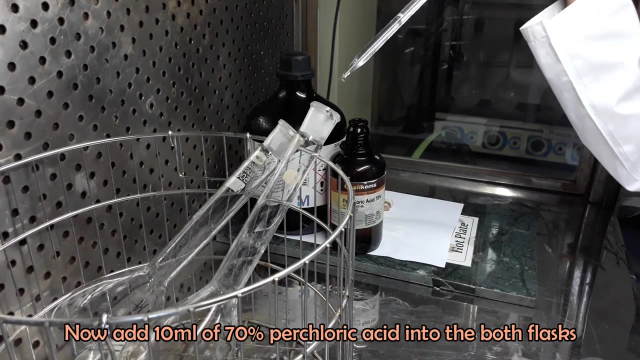 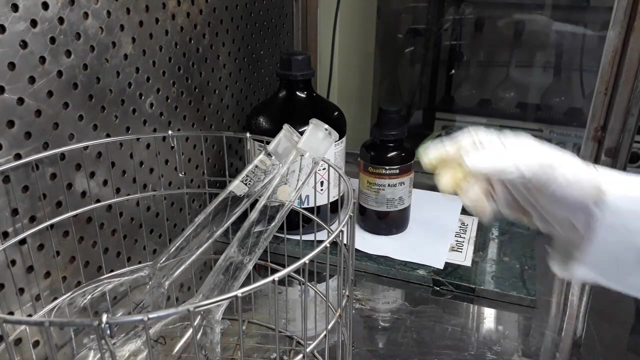 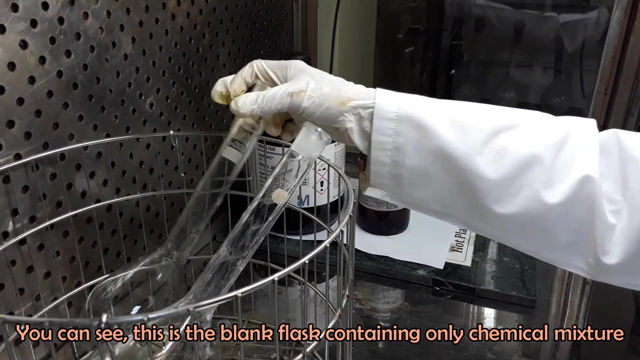 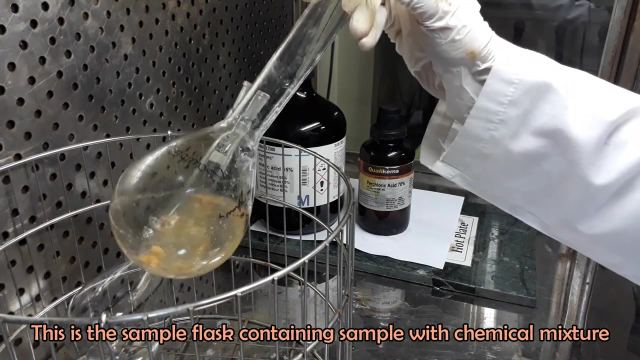 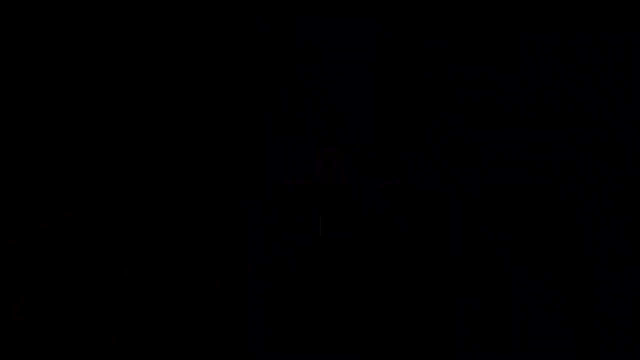 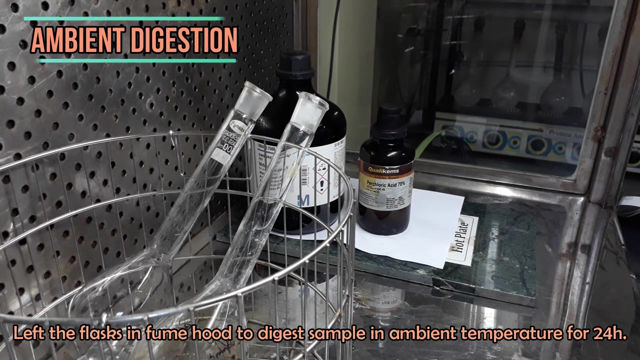 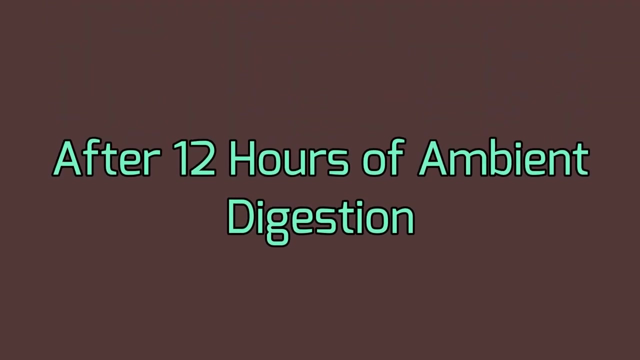 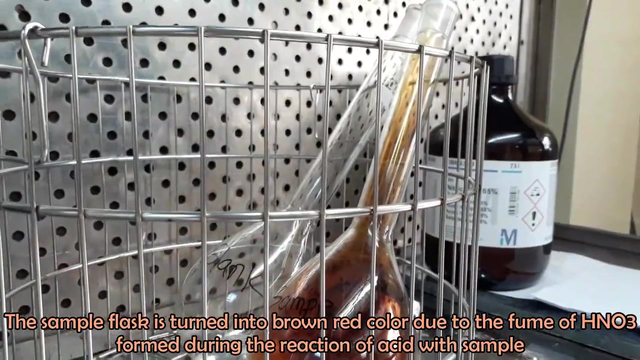 Add 10 ml of 70% perchloric acid in the same way. Shake the flask slowly. Now keep the flasks in the fume hood overnight to digest the sample in ambient temperature. After 12 hours of ambient digestion, brown color is appeared in the flask containing. 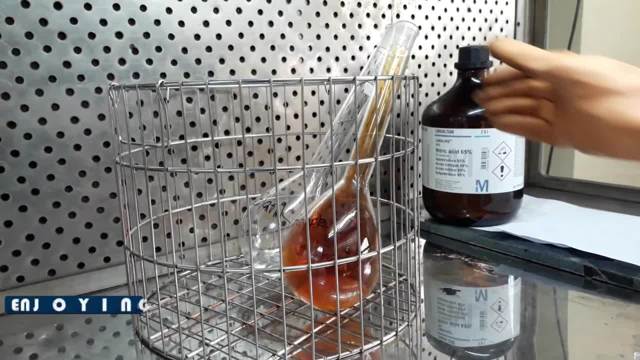 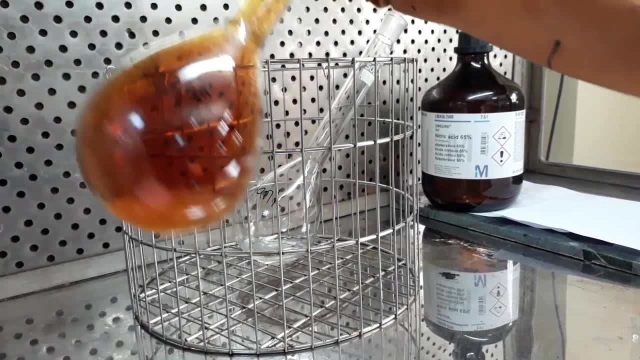 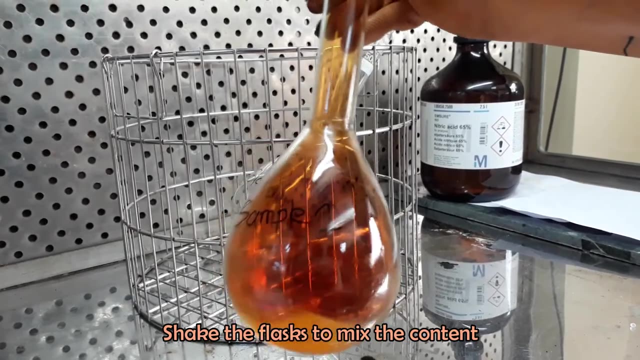 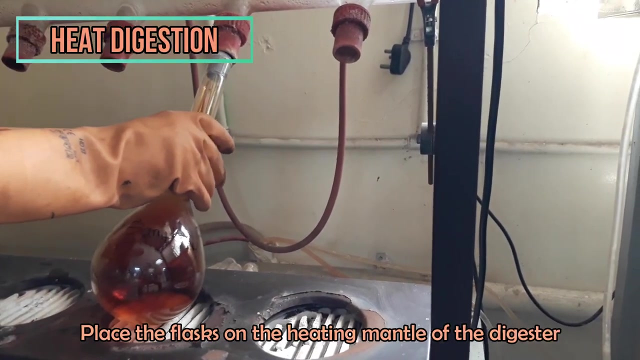 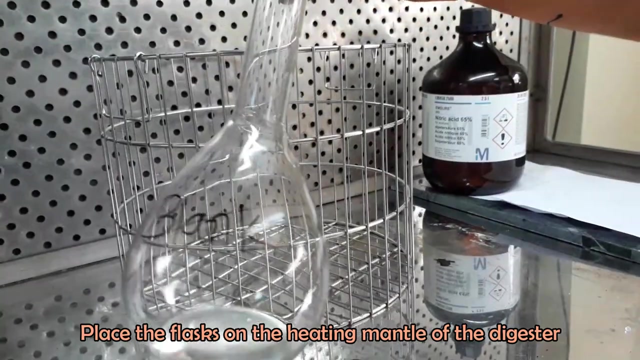 sample. This is because of the digestion of sample in nitric acid. Place the flask on a heating mantle and heat at 120 내려C節目 for heat digestion. Refrigerate the flask for 3 hours. Remove the flask fog. 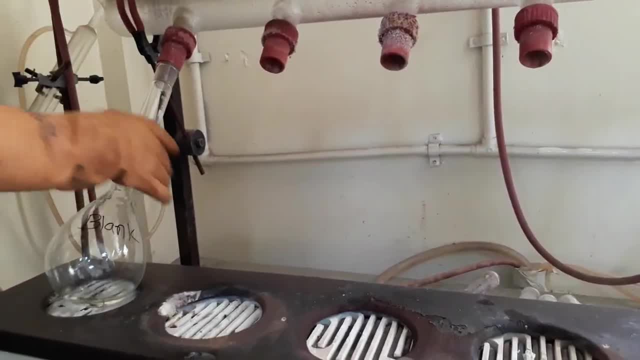 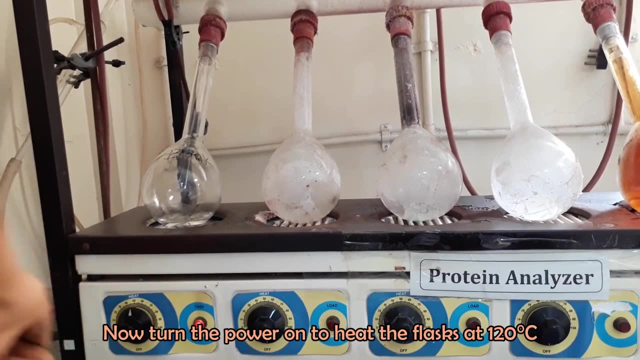 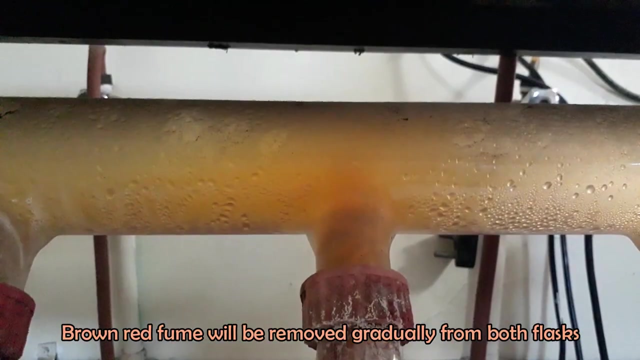 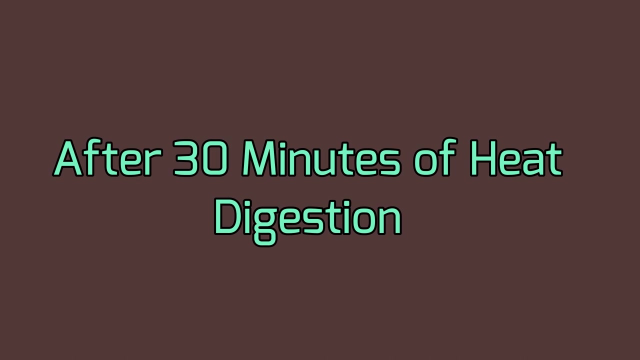 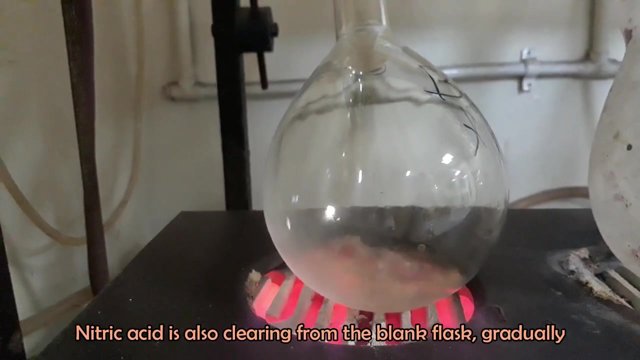 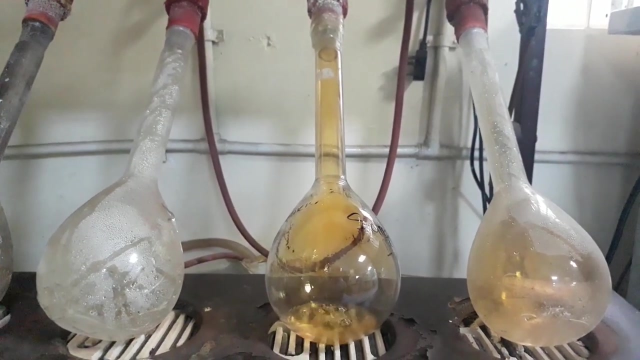 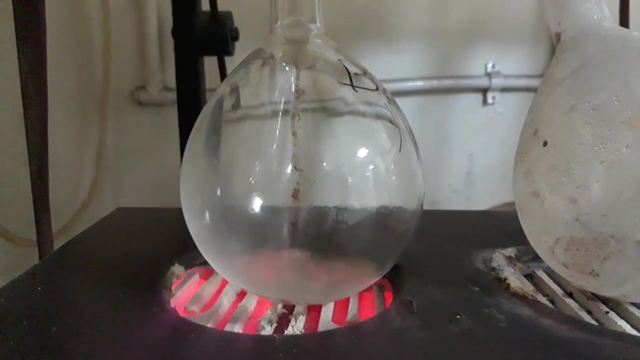 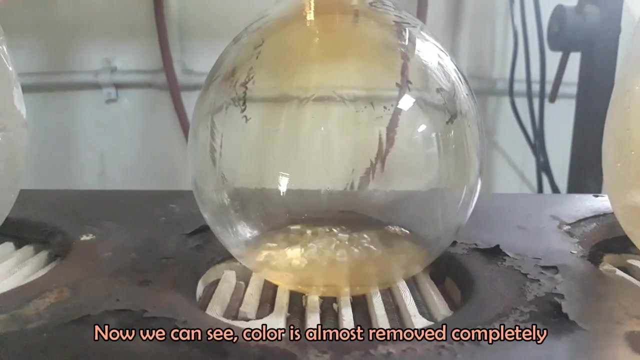 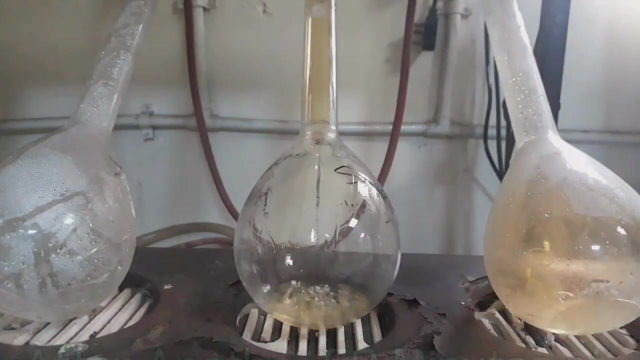 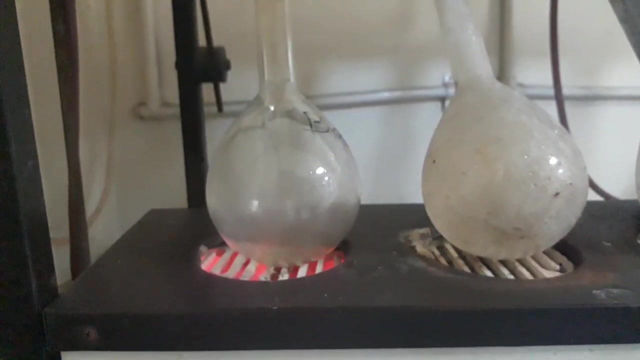 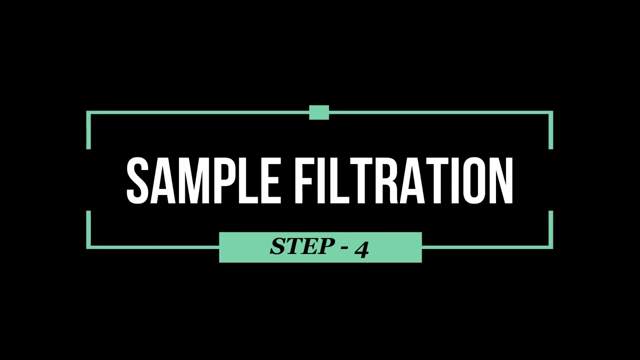 Brown-red fume is formed because of nitric acid. Brown-red fume is clearing out with time. This indicates that nitric acid is removing from the flask. Turn off the digestion when 5-10 ml of digestive juice is left in the flask. 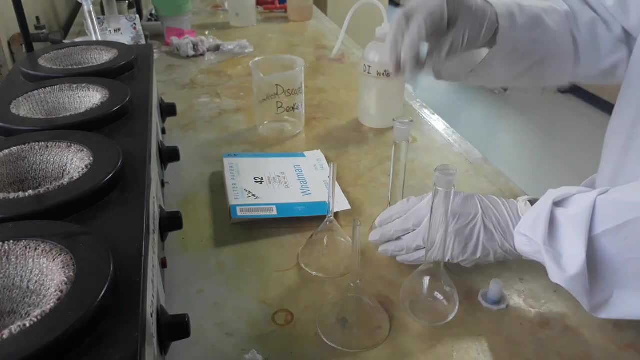 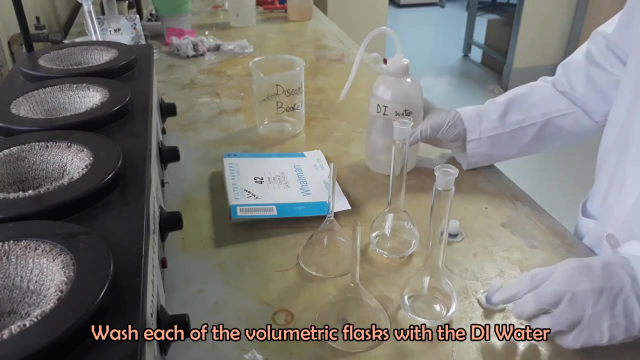 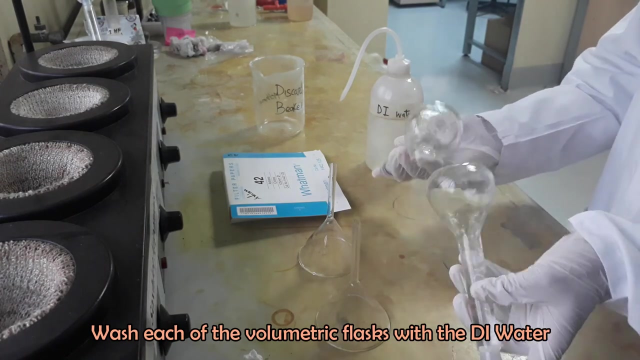 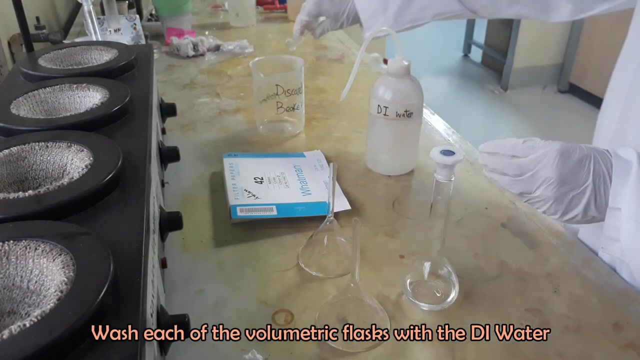 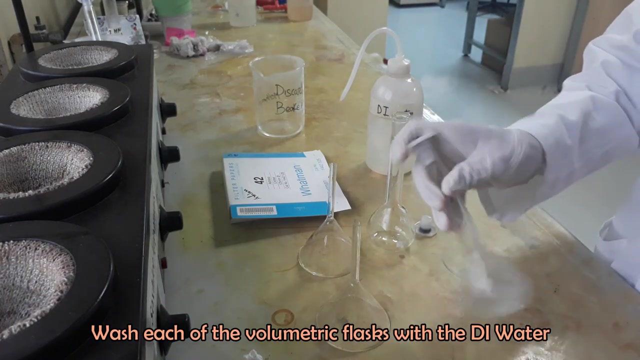 We will use deionized water to dilute the sample. Wash each of the volumetric flasks with diluent. I'll stage 3 of this辦法 before opening it. The first step, isicas brutus. We will use extractive Regionalgia guysUsine 40,As s usine 40 different劫 of Pulsanus. 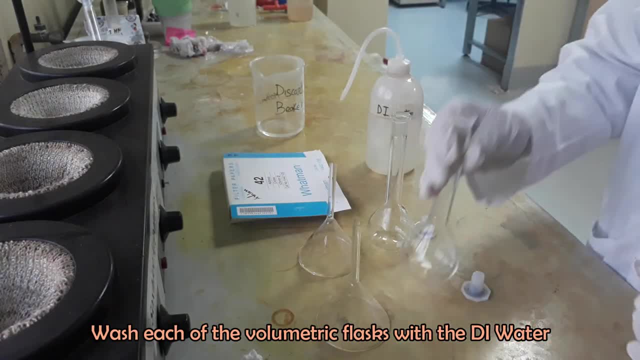 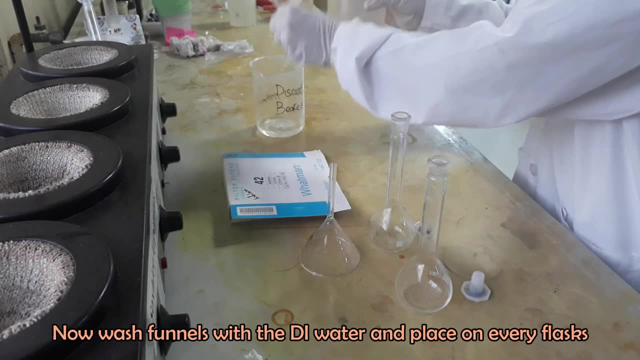 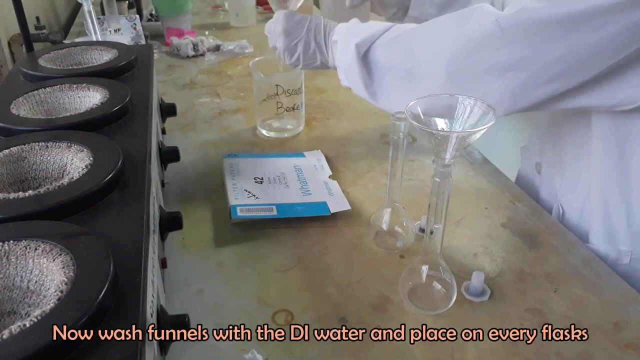 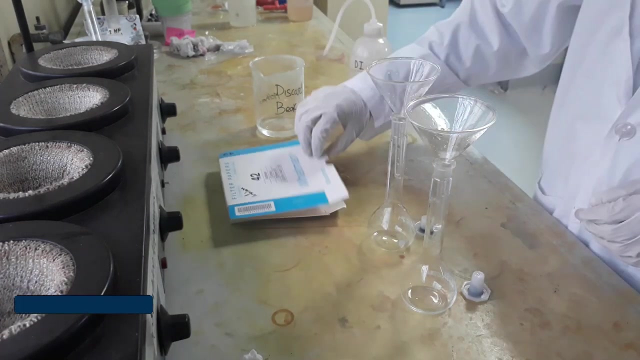 We should remove just a tiny ginseng root on the bottomthen myxxtor or aphidol phyton. Now wash all the funnels, Set aside, Repeat, Repeat the deionized water and place on every flask. 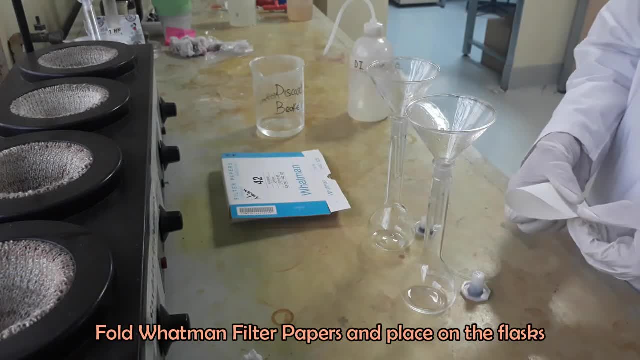 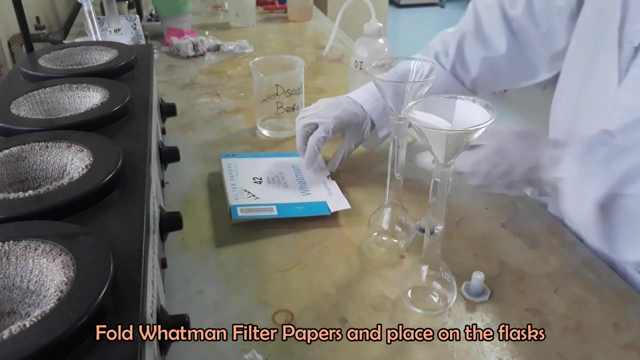 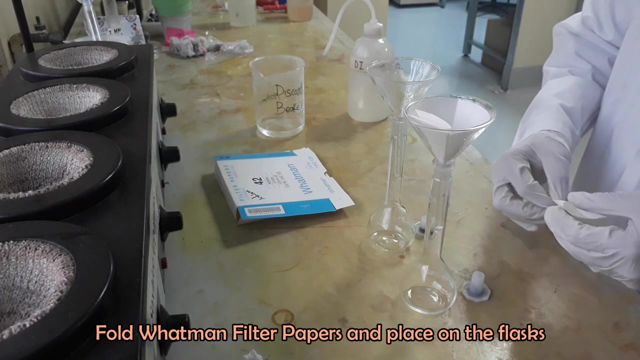 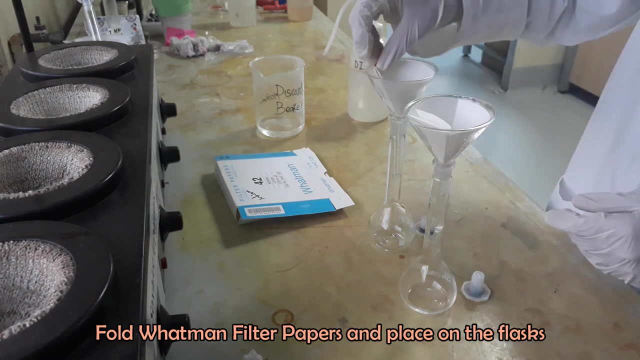 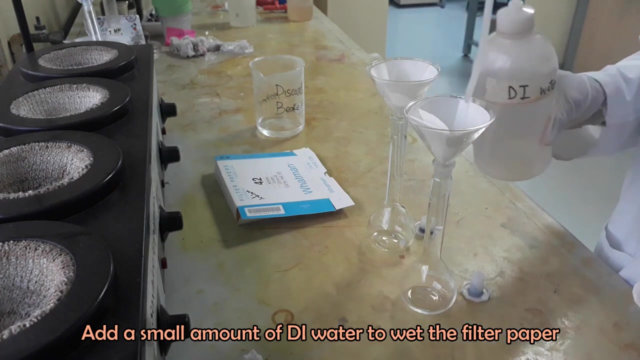 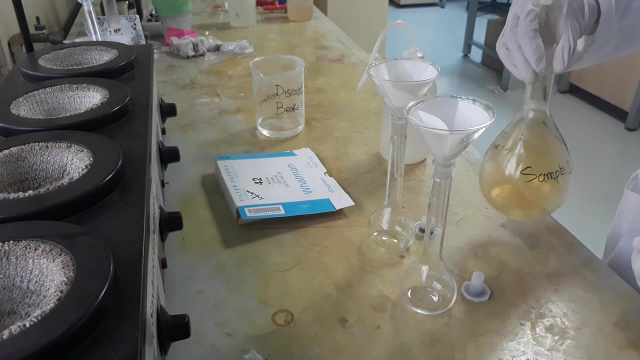 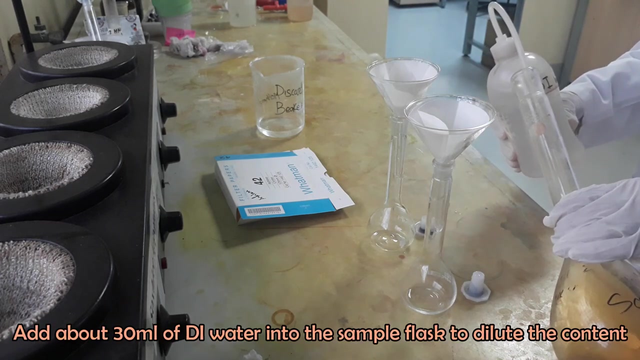 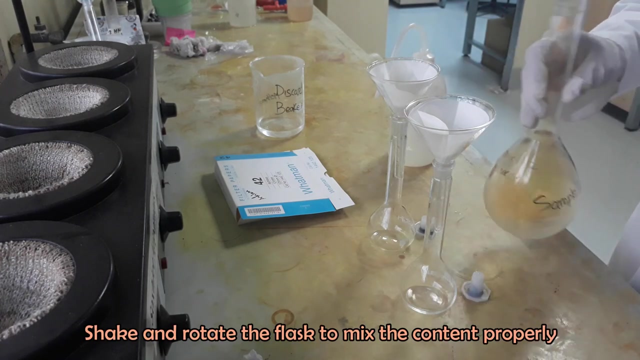 Now fold waterman filter papers and place on the funnels Pour small amount of deionized water. to wet the filter paper, Pour about 30 ml of the deionized water into sample flask. Rotate and shake the flask to mix the water well. 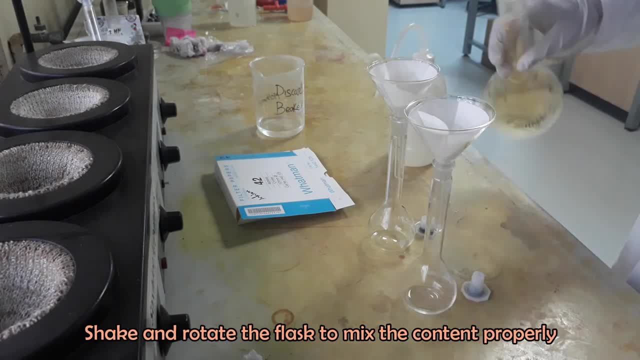 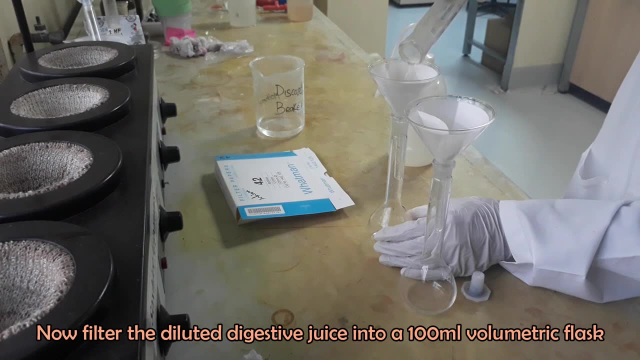 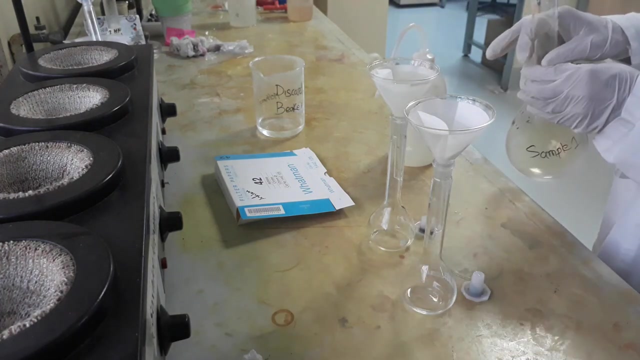 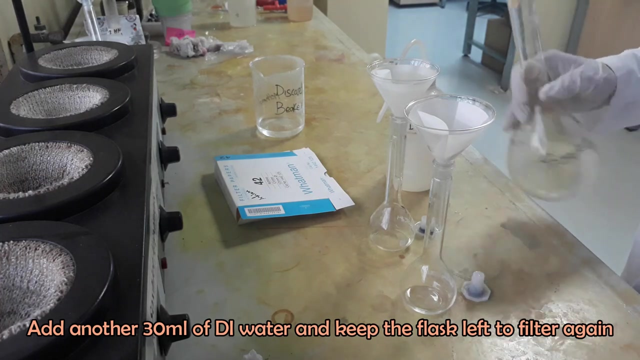 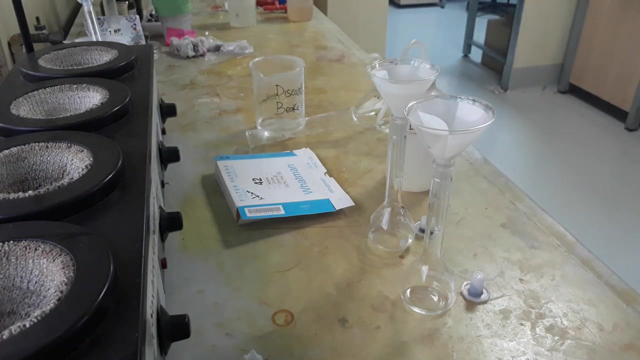 Fill the flask with digestive juice. Now filter the solution into the volumetric flask. Dip in your favoriteκαction and pour the liquid into the flask. Now filter the blank digestive juice in the same way. This will be the result of filtering. 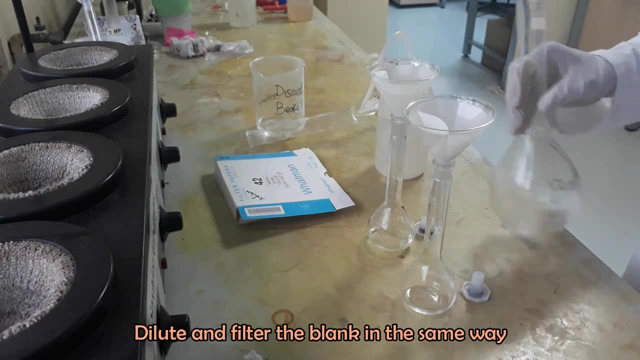 Water is much more efficient and it is a good solution. In the same way, filter the sauce. Pour the mixture onto a glass of beer. Pour 2 cups of juice into the blanched glass. Now pour the mixture onto a glass bottle. 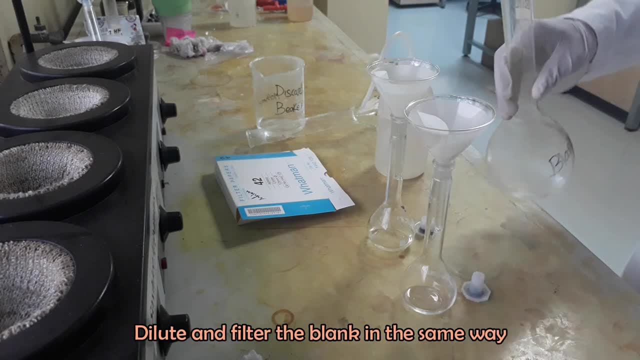 Drink this juice before serving. Drink one more glass of beer. Drink two cups of beer. Drink the remaining drink. Drink another one. Drink two cups of beer. Drink two cups of water. Drink two cups of water. Drink three cups of liquor. 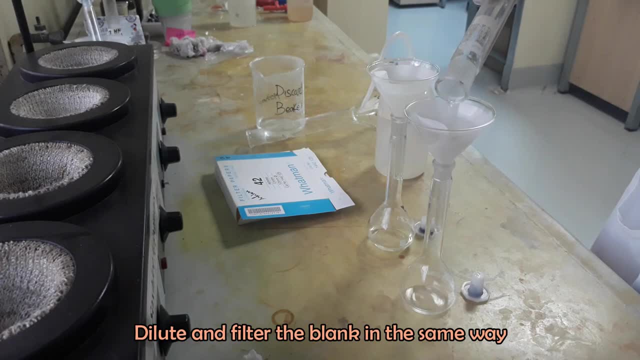 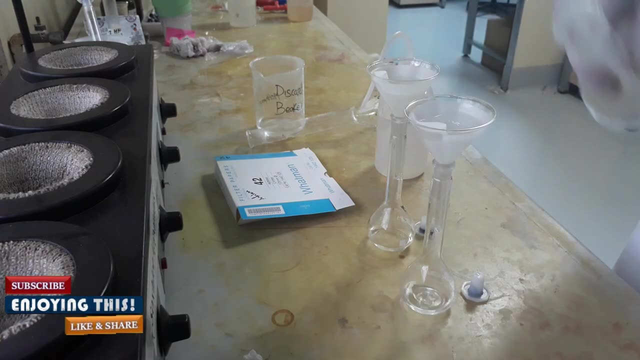 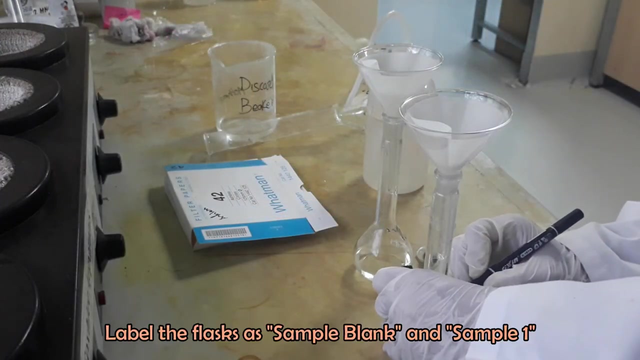 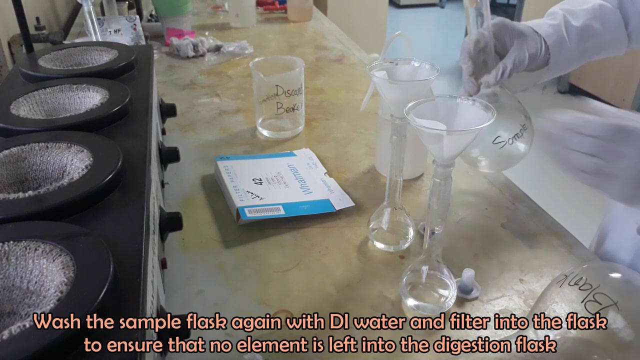 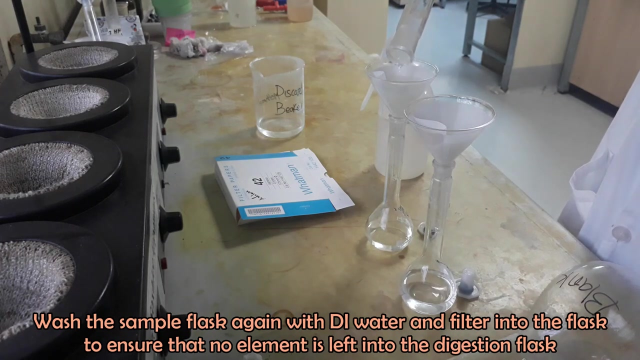 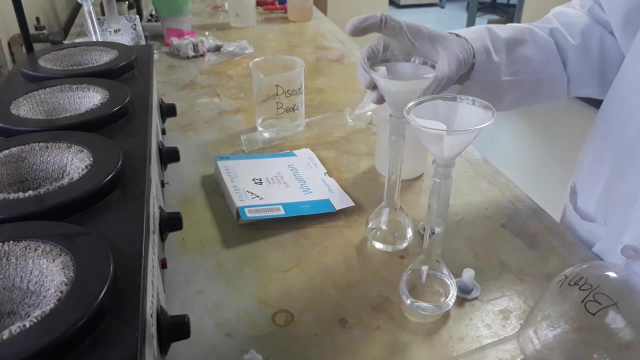 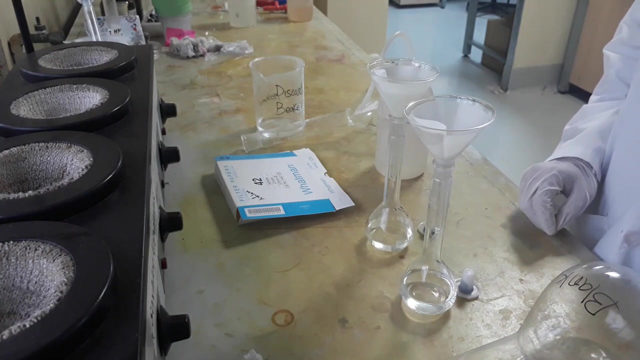 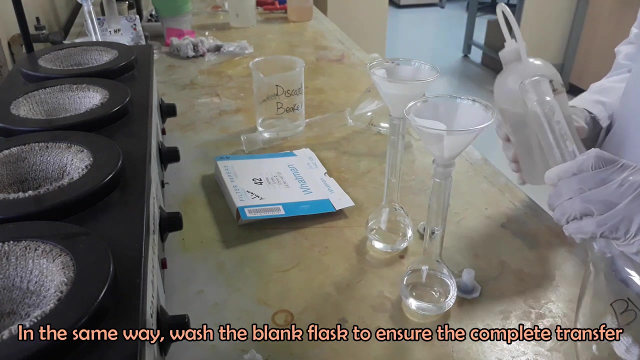 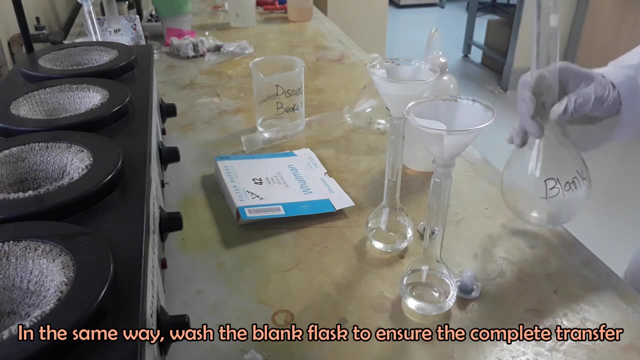 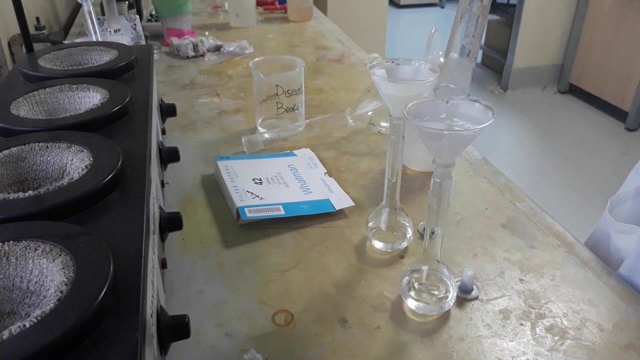 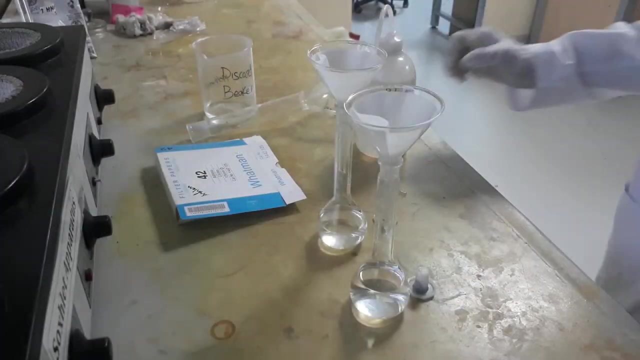 Drink two cups of water, Thank you. Add few more water into the flasks and filter again. This ensures that no element is left in the flask. Make sure that no element is left in the flask. Add some amount of deionized water washing the filter paper. 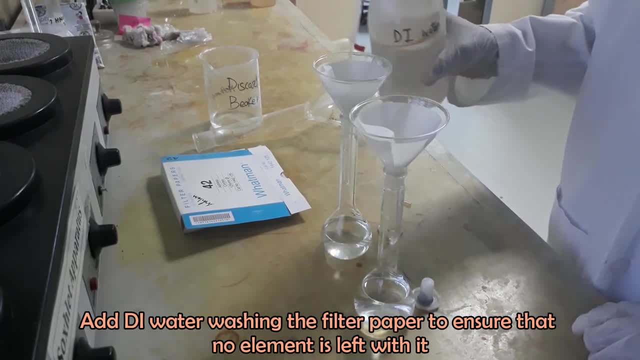 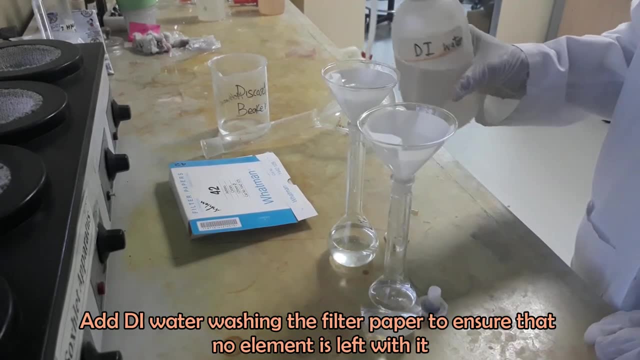 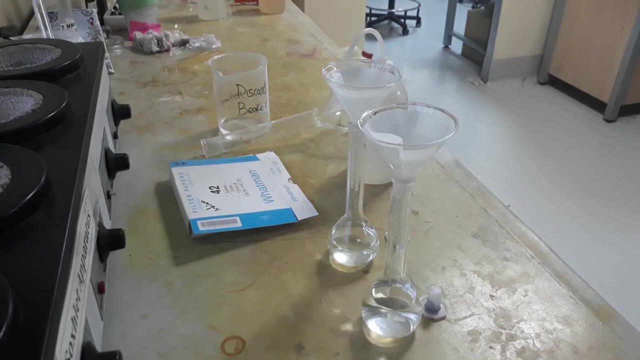 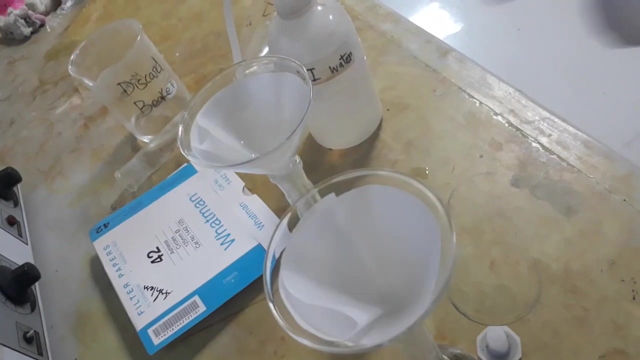 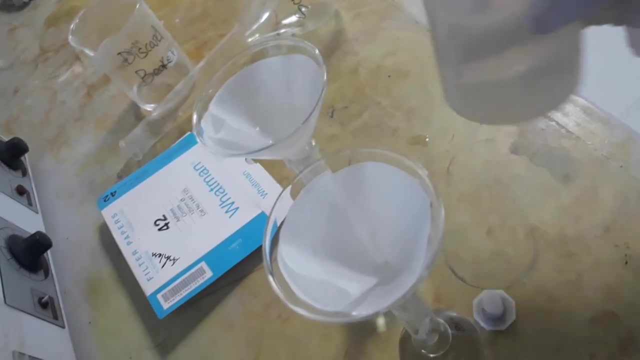 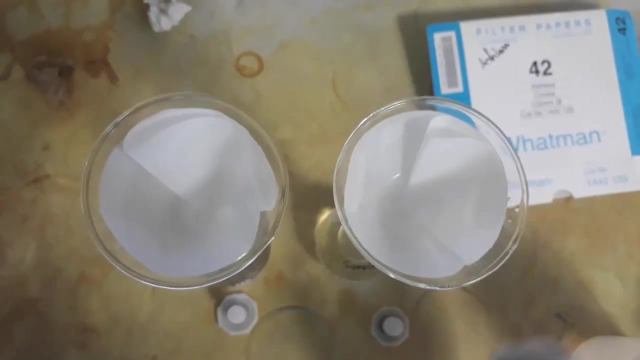 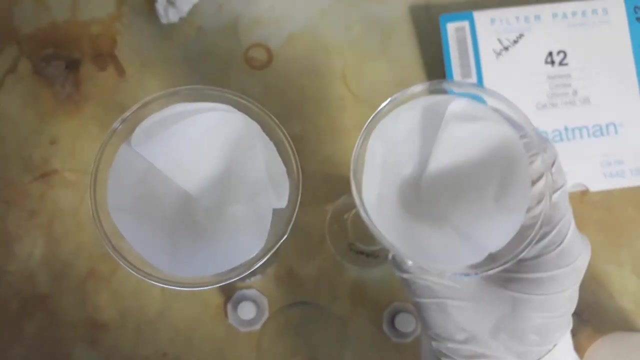 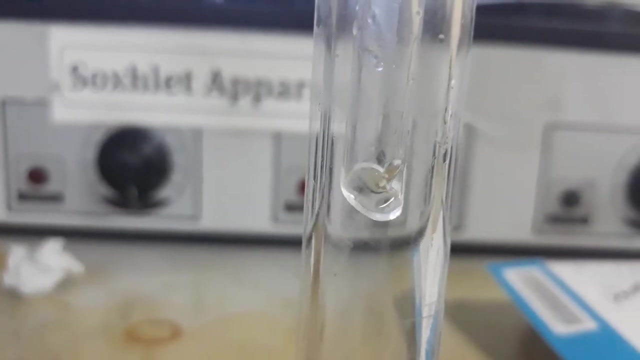 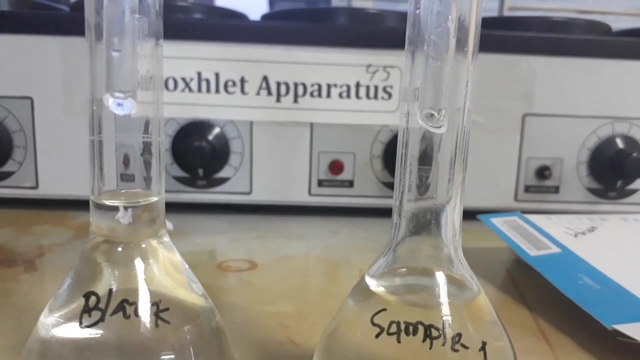 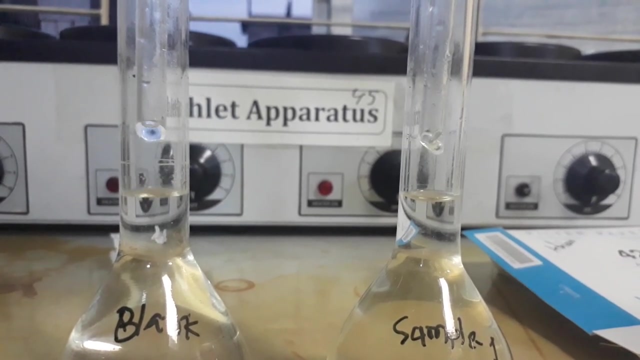 to ensure that no element is left in the flask. Add some amount of deionized water washing the filter paper. This ensures that no element is left in the flask. Add some amount of deionized water washing the filter paper to ensure that no element is left in the flask. 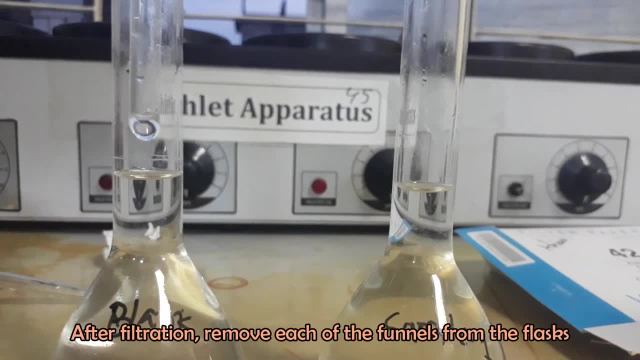 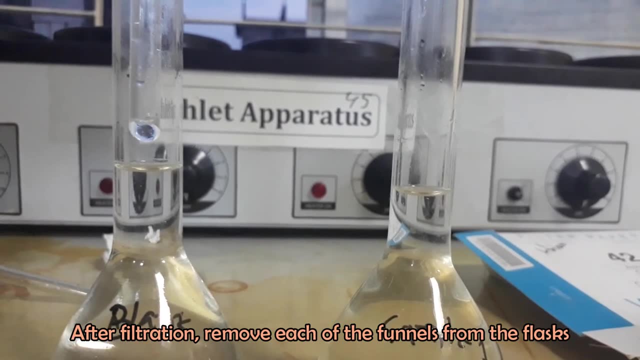 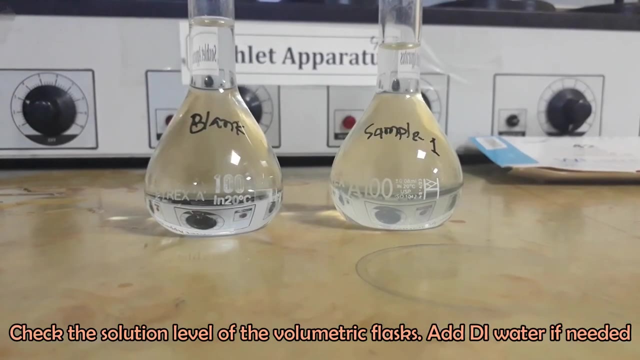 After filtration, remove each of the funnels, Take the solution level of the volumetric flasks, Level up to the mark with diluent if needed. Our sample is now ready for the analysis in AAS. Our sample is now ready for the analysis in AAS. 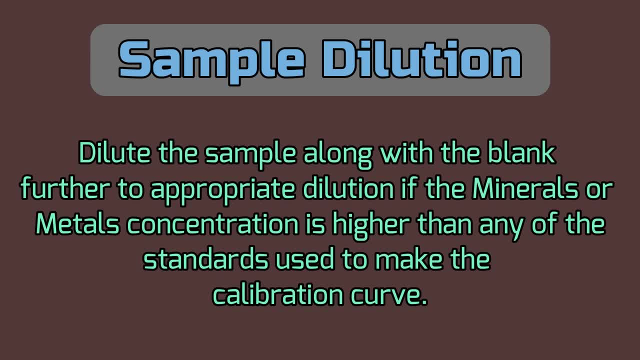 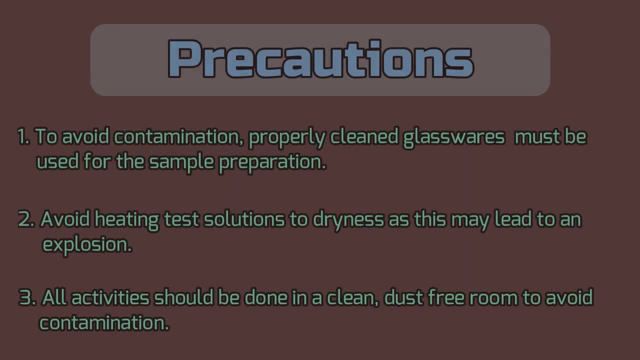 Take the sample, along with the blank, if necessary, to the appropriate dilution. if the concentration is higher than any of the standards used to make the calibration curve, Some precautions should be followed to throughout the sample preparation. They are to avoid contamination. properly cleaned glassware must be used for the sample preparation. 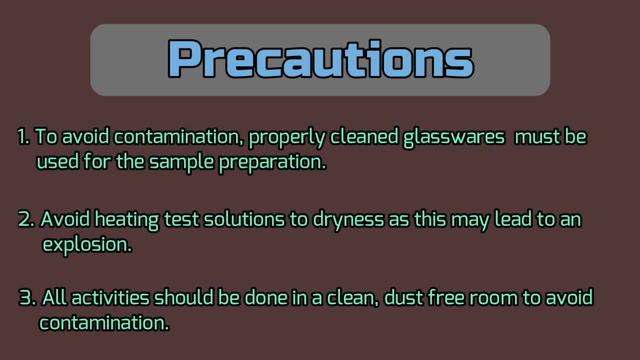 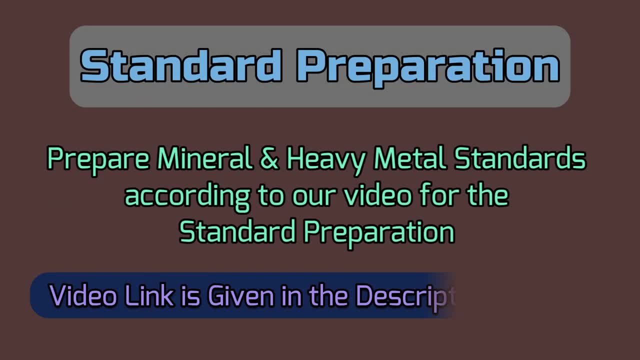 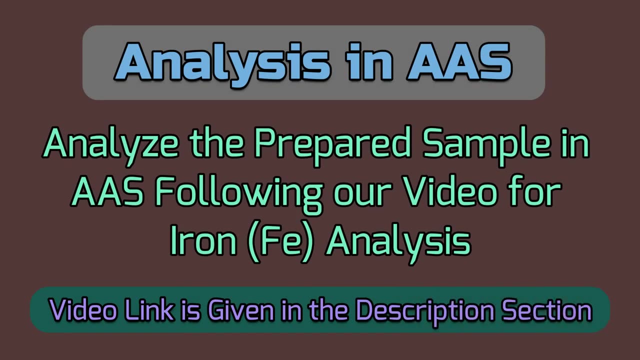 Avoid heating test solutions to dryness, as this may lead to an explosion. All activities should be done in a clean, dust-free room to avoid contamination. Prepare mineral and heavy metals. Prepare mineral and heavy metals according to our video for the standard preparation and analyze the prepared sample in AAS, following our video for the iron analysis. 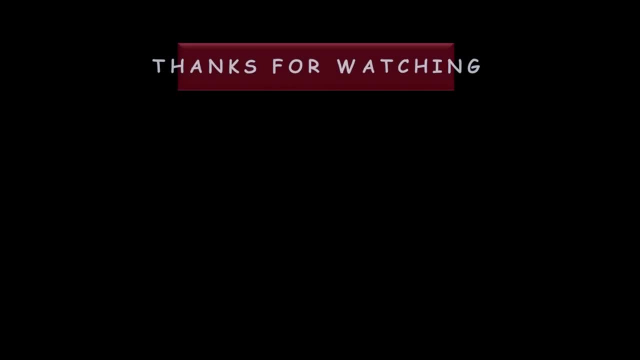 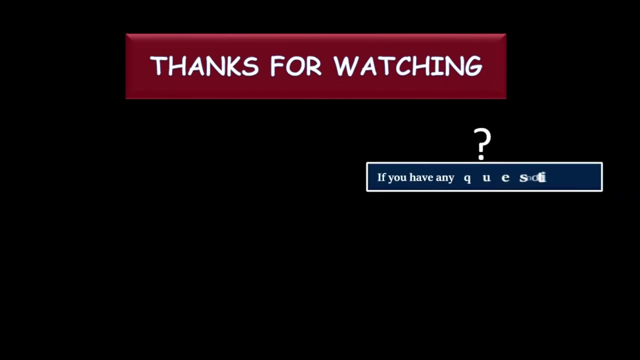 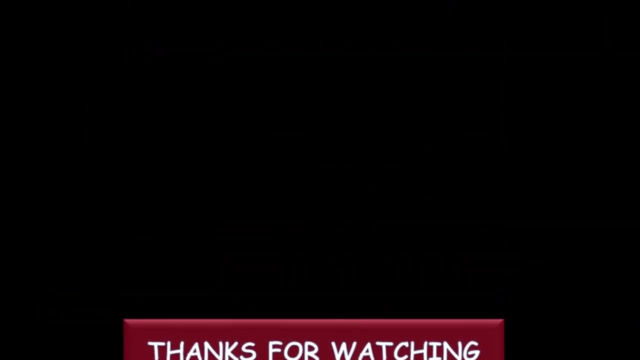 Video links are given in the description section. Video links are given in the description section.